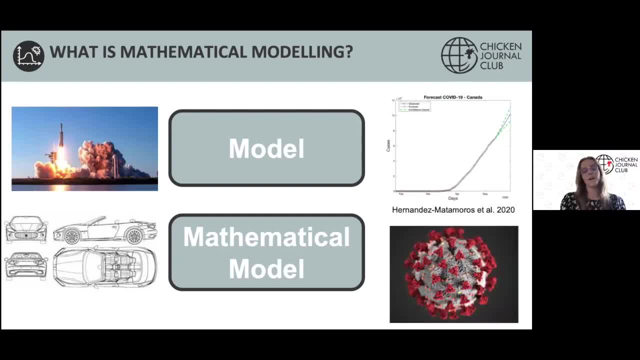 quite a lot of these models for the COVID pandemic, where, for example, here we have real life data, day to day data on the cases in this is COVID-19 cases in Germany and cases in Canada, And so we can see how this progresses. then they use this data to forecast. 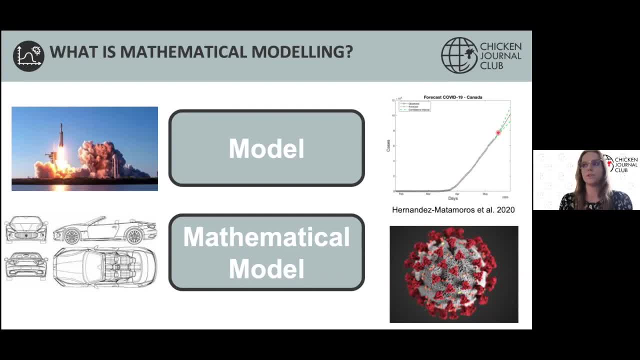 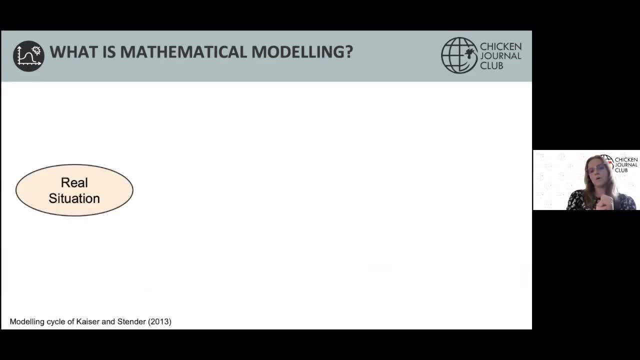 which is this black line here- with confidence intervals using mathematical models. So, COVID-19 and mathematical modelling: How do we build our mathematical models? So this is a modelling cycle from a paper in 2013, where they defined how to do this. So you start with your real 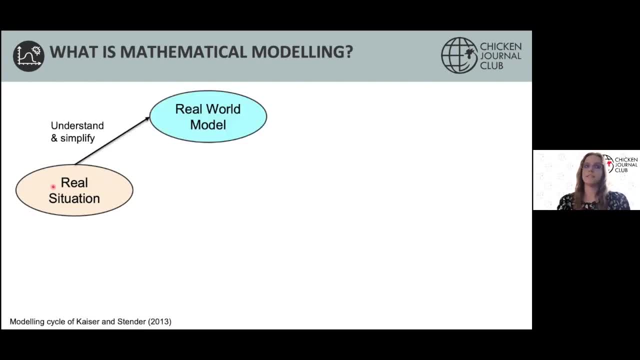 life situation Which you can understand and simplify to build this real world model. From this. you then use mathematical concepts and languages to build your mathematical model, Which you then conduct. so obviously this is quite a simplified thing. so you conduct the mathematical work to get this mathematical result from this, Which you then interpret. 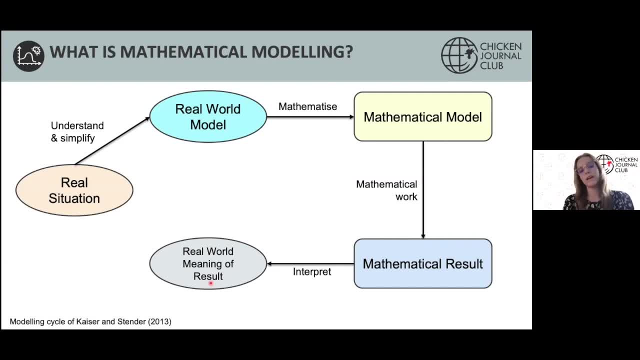 to get real world meaning of these mathematical results. This can then go one of two ways. You validate your model. it fits your real life situation, which is perfect. you've now got a model which fits your real life data. or you actually find that, once you validate, you actually don't hit your real life situation. 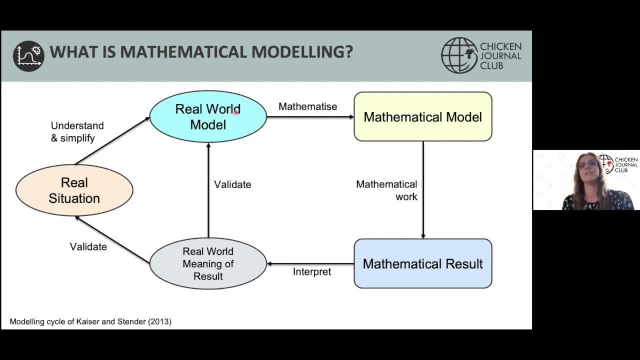 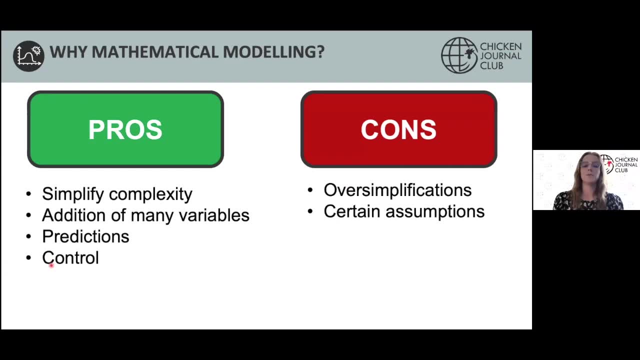 so you go back to your original model. do this loop again until you actually find something which fits your real life data. pros and cons of mathematical modeling. mathematical modeling allows you to simplify something which is complex and might be costly or not time effective. you can add many variables um at different stages, so you can go back to your basic model and add variables. 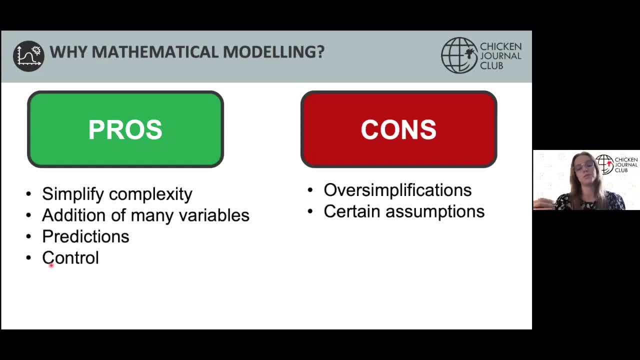 as you go along. it allows you to make predictions for future events without them actually occurring, and you can see different control measures to change the predictions that you've got within your model. however, you can sometimes oversimplify your model, so what you've actually predicted doesn't fit real life situations, and sometimes these models only work under certain assumptions. 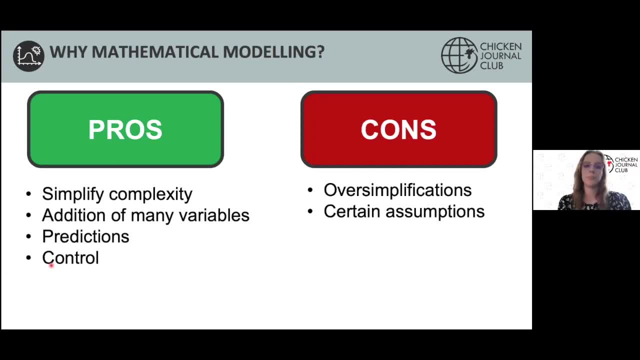 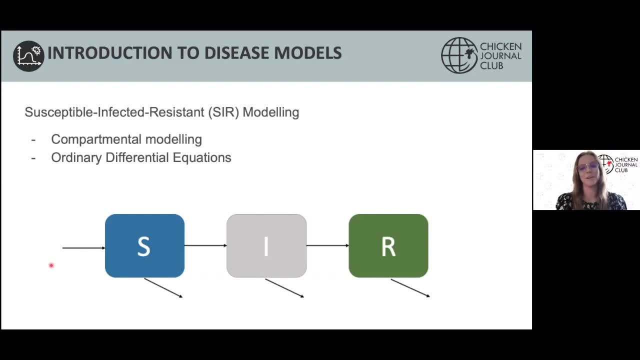 which aren't realistic for real world situations. so introduction to disease models: you've probably all heard about sir models by now with the current pandemic, and so these are susceptible infected resistance models which basically takes a population level approach and takes all the individuals and places them into 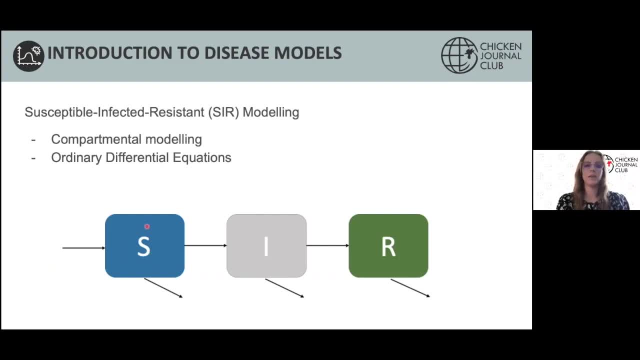 one of, in this instance, three compartments which we have- the susceptible, infected and resistance compartments- and it uses the parameters here to form ordinary differential equations which i'll go into later on in the presentation. examples of sir models are measles. this is quite a common one, one of the early. 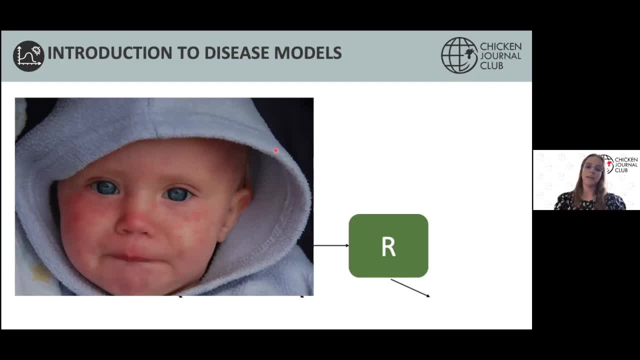 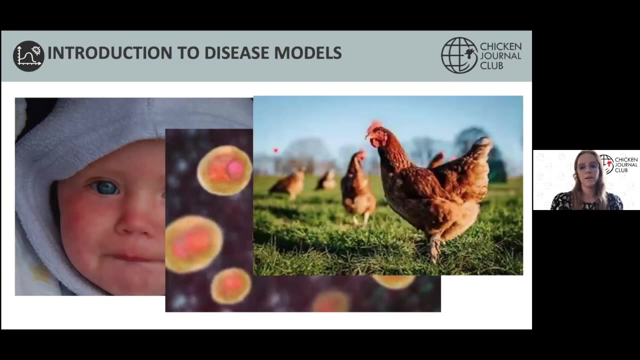 sir models to be developed. the sir model here was helped with the vaccination program and it also looked at age dependencies of infectious diseases, sexually transmitted diseases, which have a heavy focus on contact tracing. but what about in poultry? how can we use sir models within a poultry setting? 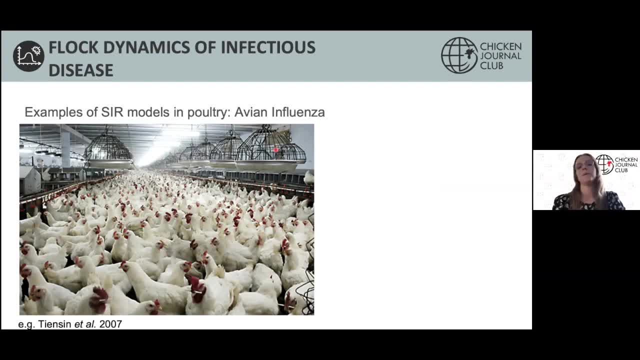 so take a flock, for example. so flock dynamics of infectious diseases. this is an example with avian influenza. so take your population of chickens. um, all of these chickens are susceptible at the moment. they're in our susceptible compartment of our sir model and you have some kind of external force of infection. so they're susceptible to the infection of the poultry. but 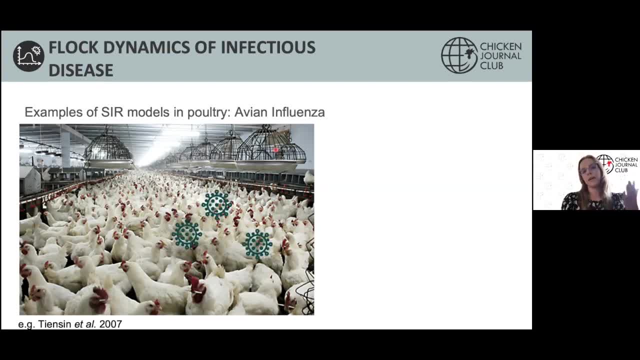 which brings avian influenza into our flock. This then spreads around the flock. as all of our chickens are deemed to be susceptible at this current moment in time, What do we want to know? We want to know the transmission parameter, beta. We want to know the force of infection that is. 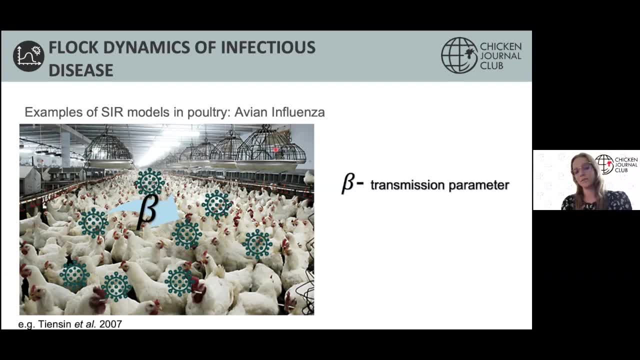 causing these chickens to go from the susceptible compartment into the infected compartment. From this we also want to know what is the reproduction number, or R0.. So R0 is the expected number of secondary cases produced by a typical primary case in an entirely susceptible population. 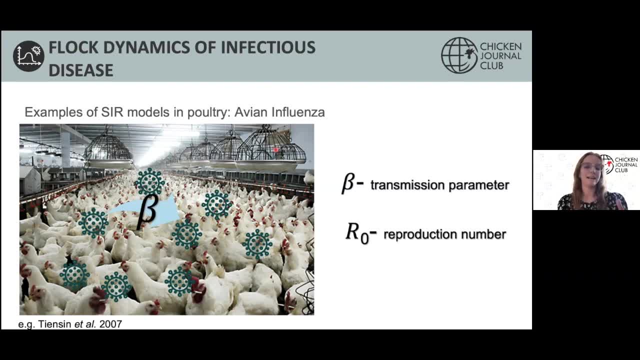 such as our chickens. This R0 value has a threshold value, so within the past year there's been a big emphasis on what the R0 number is of COVID-19.. If this R0 number is greater than one, the disease will continue to spread. If this R0 is less than one, the transmission will fade. 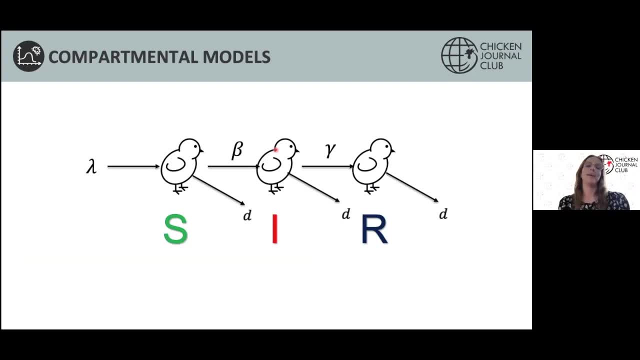 So this brings us to our compartmental models. So here I've represented our compartments by these three little chicks. So we have susceptible individuals, infected individuals and recovered individuals. We have different parameters. So here lambda represents the number of births into our system, D is the mortality coming out of our system and we have the force of infection and the recovery. 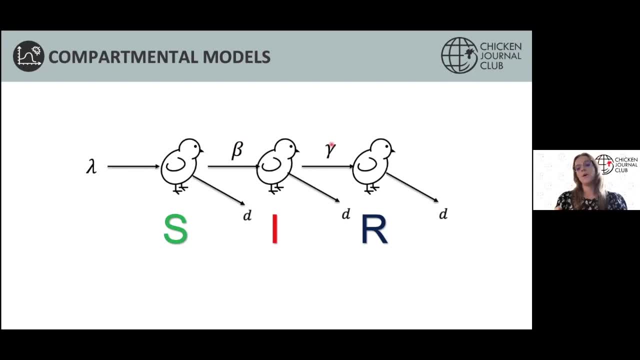 rate, So we can see that our population is really close to the normal rate of our population. Within a chicken flock is very likely to be a closed situation, so we're not going to have our births or death rates but for simplicity, I'm going to keep these in our model. 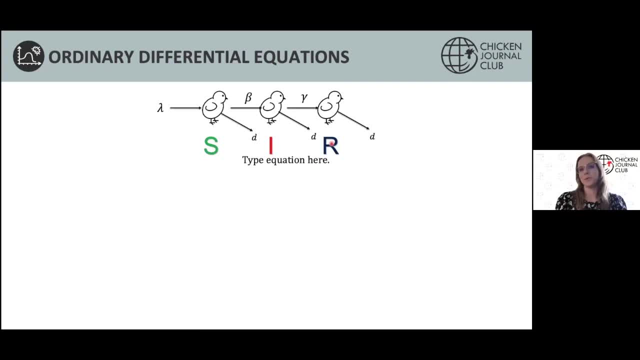 From this we can build our ordinary differential equations. So that type of equation here is not supposed to be there. So we have our equations, which look something like this: So don't be put off, this is quite simple. So we have our change in susceptible. 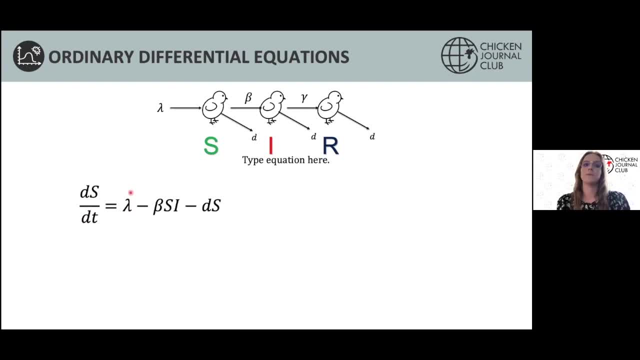 change in time. So how does our susceptible compartment change over time? So we have our births going into our population, minus our transmission parameter and the number of times, the number of susceptible and infected, minus the mortality rate of the susceptible compartment. By building a framework like this, we use our arrows to determine whether something is going. 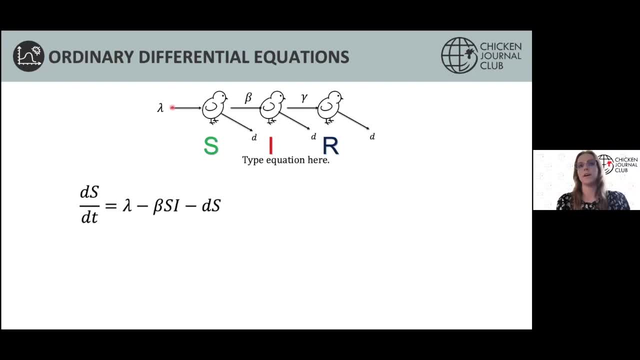 into or out of the population, So the compartment, sorry. So here we have an arrow going in, so we are adding it to our S, But these two arrows are going out, so we're taking them all in, So we're taking away. and again it's going in, so we're adding. it's going out, so we're taking it away. So, looking at, 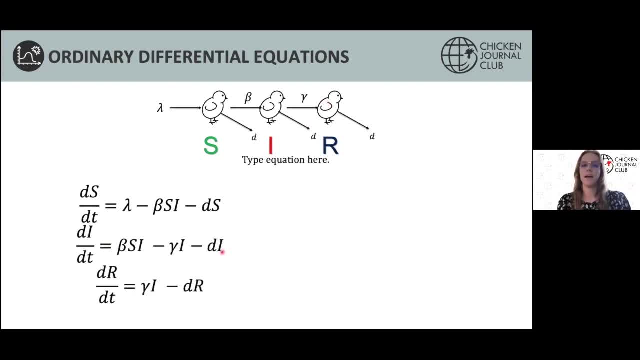 our infected individuals- we can do exactly the same here. and our recovered individuals. we can do exactly the same here, Using our SIR models. we can also work out the R0 value using our beta and recovery rate. You can enter these into any form of coding program. I use R and I use the Shiny app. 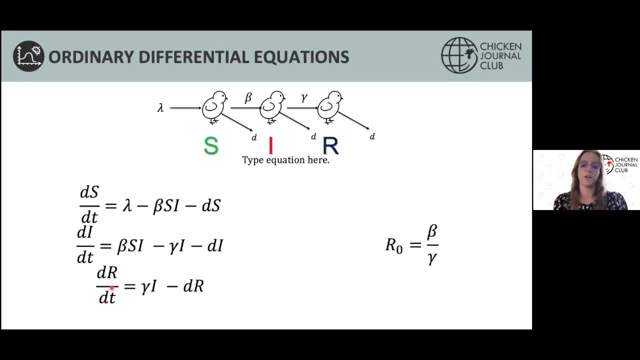 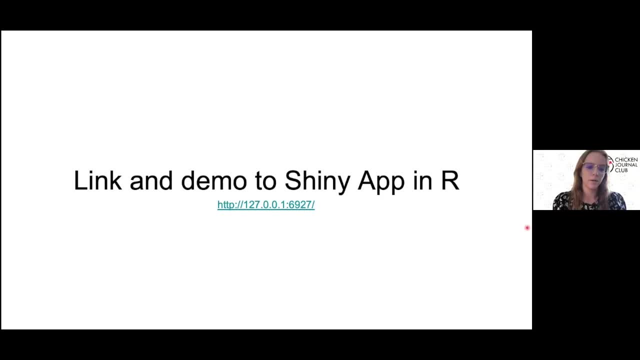 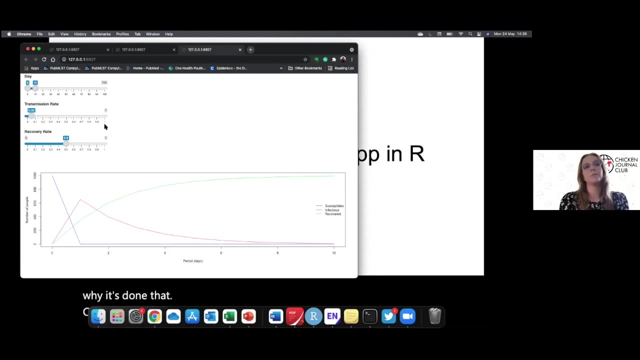 which helps me make it a little bit more interactive. So I'll show you how. a quick demo on Shiny, Let me get my mouse back. So here we have our Shiny app, which allows us to change, for example, the number of days in which we 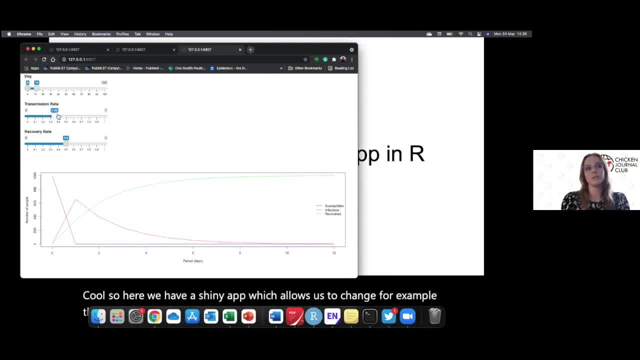 want to have our system running for our transmission rate, which we can increase or decrease, and our recovery rate, Which we can increase, decrease, and here it will show the change in susceptibles, infected and recovered individuals over time. You can add different variations of this as you wish. 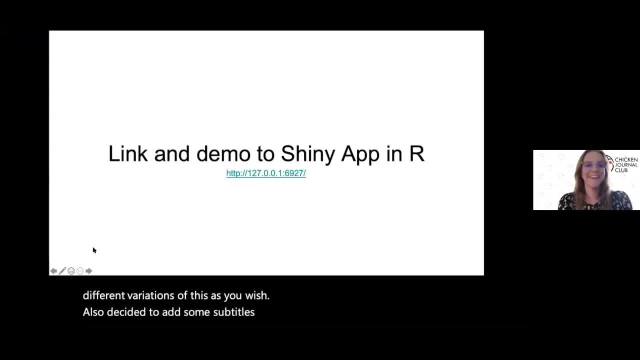 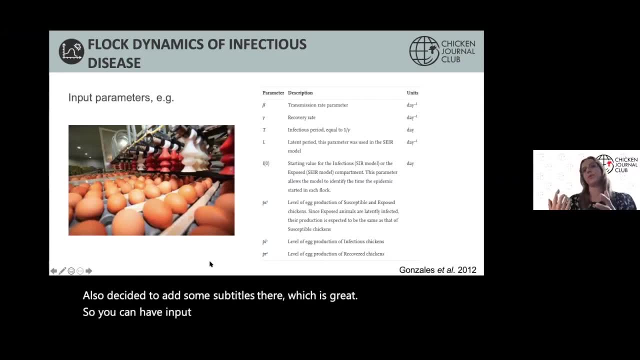 It's also decided to add some subtitles there, which is great, So you can have input parameters into your model. So you typically set up a table which looks like this, So you'd have your parameter down the side: the distribution, the number of days, the number of days, the number of. 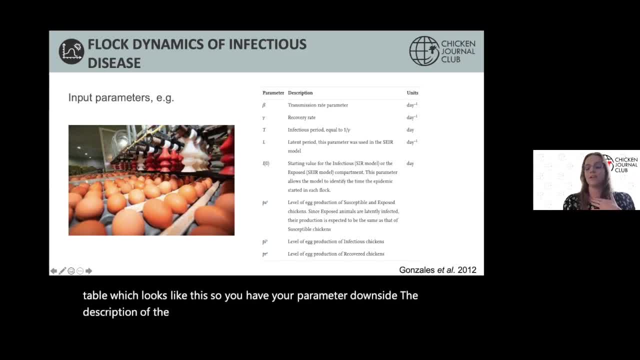 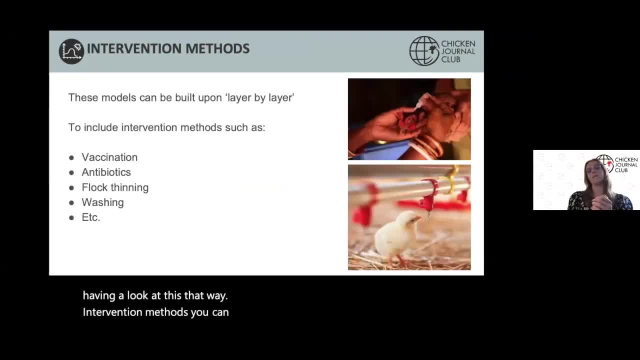 Intervention methods. You can build upon these methods. these models are layer by layer to have a look at how intervention methods would likely change the prevalence of disease at the end of the flock cycle. So you can include intervention methods such as vaccination antibiotics which 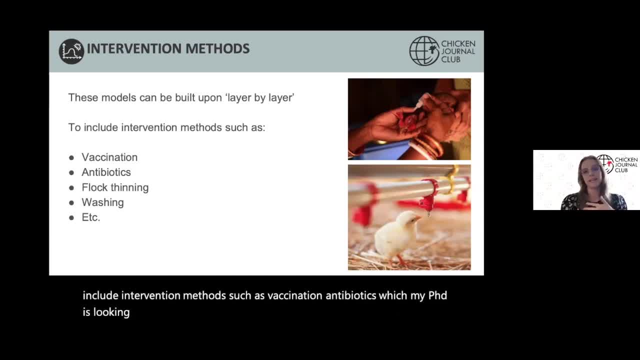 my PhD is looking at. You can also include intervention methods such as vaccination, antibiotics, which my PhD is looking at- Flock thinning, washing, all kinds of different things which may be costly and timely, but if you model it, it's not going to take that long. 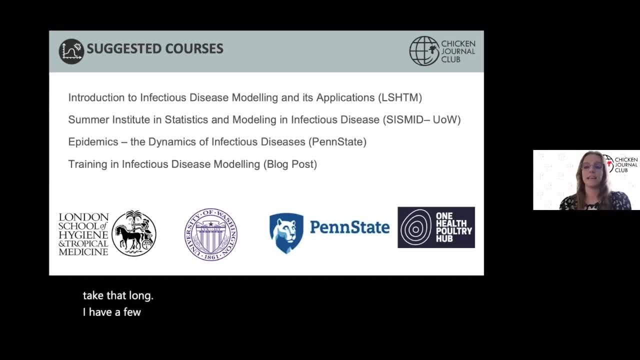 I have a few suggested courses if you're interested in getting into infectious disease modelling. So there's an introduction to infectious disease modelling by the London School of Hygiene and Tropical Medicine which is in June. I did this last year and it really helped me with the basics. 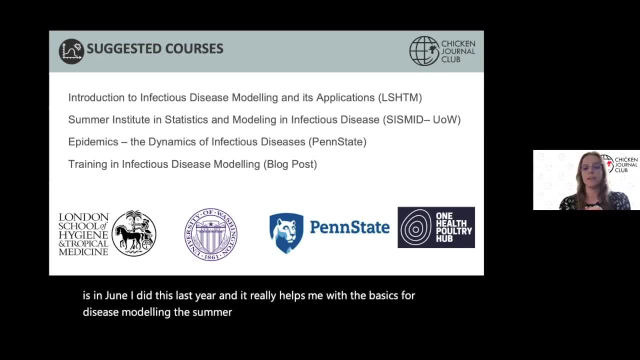 for disease modelling, So I'm going to talk a little bit more about the basics of disease modelling, The Summit Institute of Statistics and Modelling Infectious Diseases by the University of Washington. I'm using that in a couple of months time to help me with data fitting to my models.